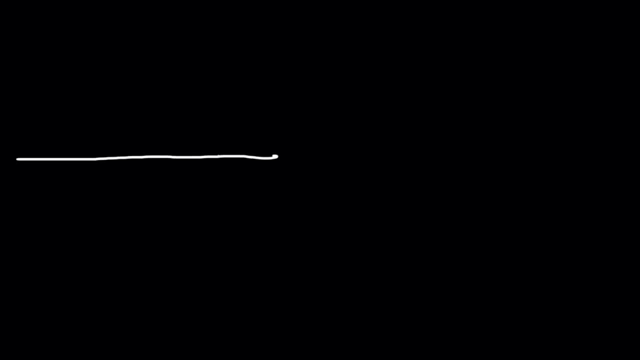 Now let's talk about how to find the value of a limit from a graph. Let's just make some points first. So let's say, if we have an open circle at this point, a closed circle and also another open circle, What is the limit as X approaches? 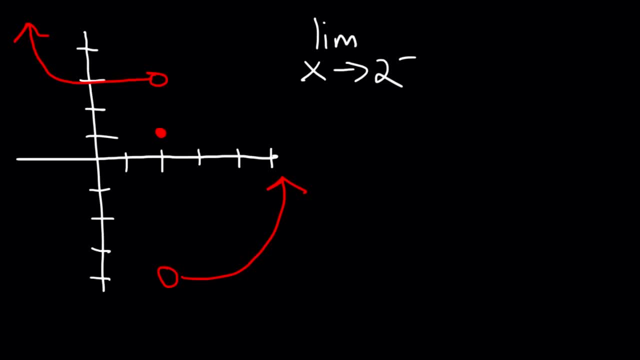 2 from the left side. So this is known as a one-sided limit. Now let's call this function f. So basically, this question is asking you: as X approaches 2 from the left, what is the y-value? So here is an x-value of 2.. As we approach it from the left side, notice: 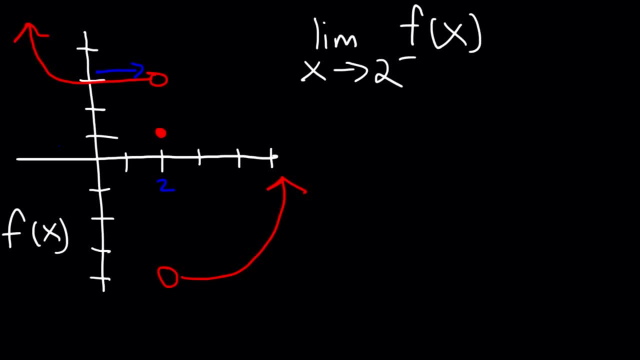 that the y-value of that curve is 3.. This is 1, 2, 3.. Now, what is the limit as X approaches 2 from the right side of f? Now, if we follow the curve from the right side as we approach an x-value of, 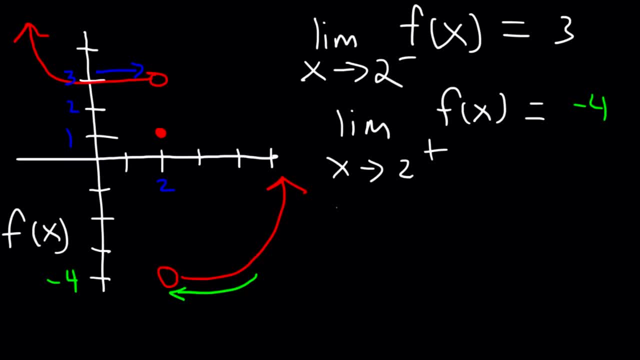 2, notice that the y-value is negative 4.. Now, how about the limit? as x approaches 2 from either side? Because the left side and the right side do not match, this limit does not exist. Now, what about the value of f? 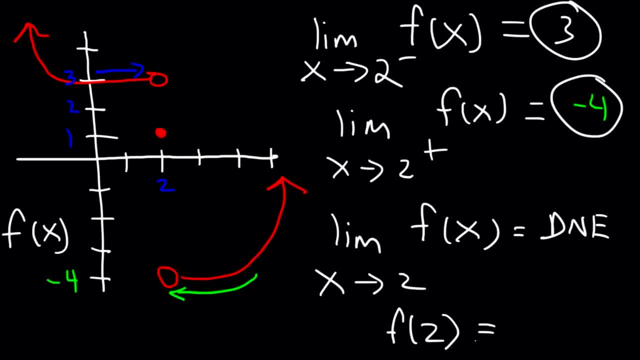 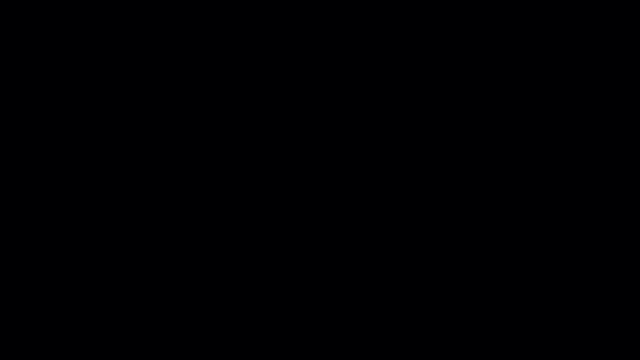 When x is exactly 2, what is the y-value? So we have to look at the closed circle. The y-value is 1, so f is equal to 1.. Now let's try another example. Let's say if we have an open circle at that point and a closed circle here, 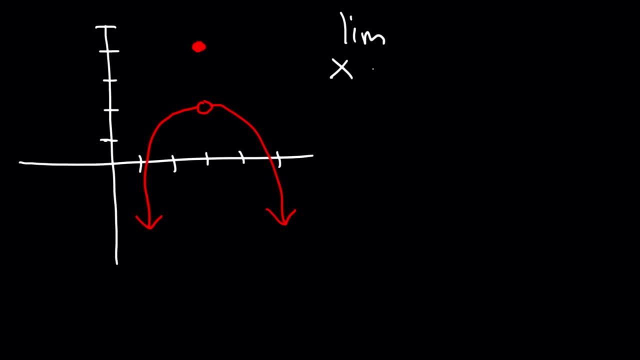 What is the limit? as x approaches positive 3 from the left side, And this is the graph of f. So here is an x-value of 3.. As we approach it from the left side, notice that the y-value is 2.. 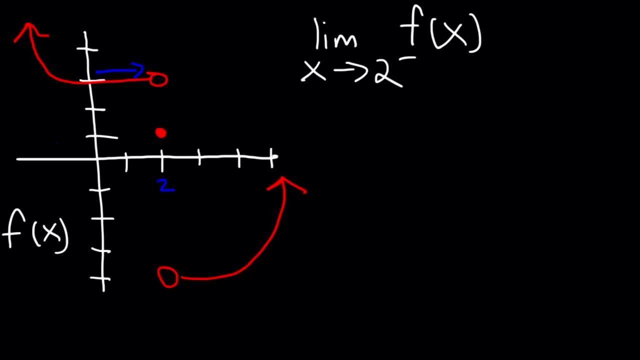 that the y-value of that curve is 3.. This is 1,, 2, 3.. Now what is the limit as X approaches 2 from the right side of f? Now, if we follow the curve from the right side as we approach an x-value of, 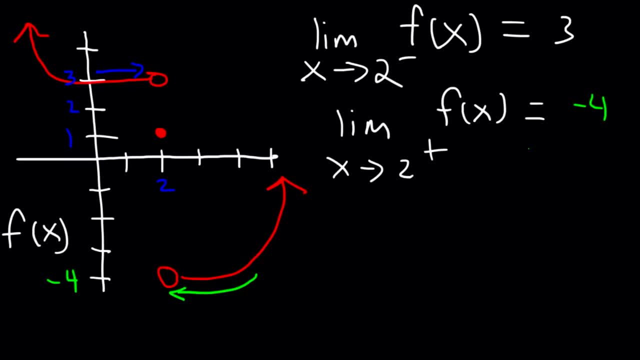 2, notice that the y-value is negative 4.. Now, how about the limit as X approaches 2 from either side? Because the left side and the right side do not match, this limit does not exist. Now, what about the value of f When x is exactly 2,? what is the y-value? So we have to look at 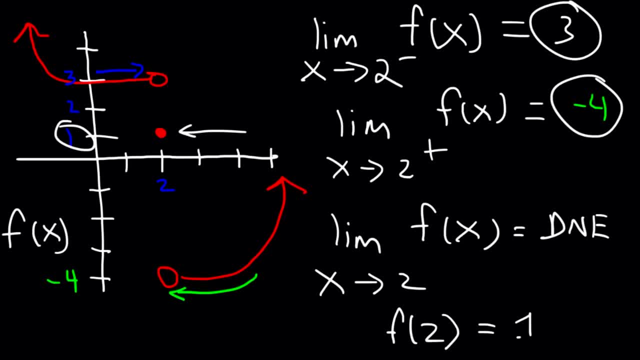 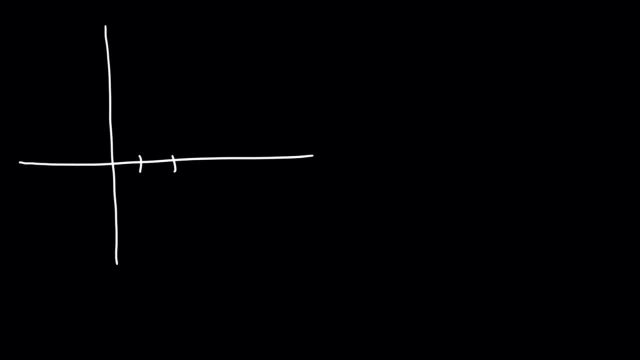 the closed circle, The y-value is 1, so f is equal to 1.. Now let's try another example. Let's say: if we have an open circle at that point and the closed circle here, what is the limit as X approaches positive 3 from the left side And this: 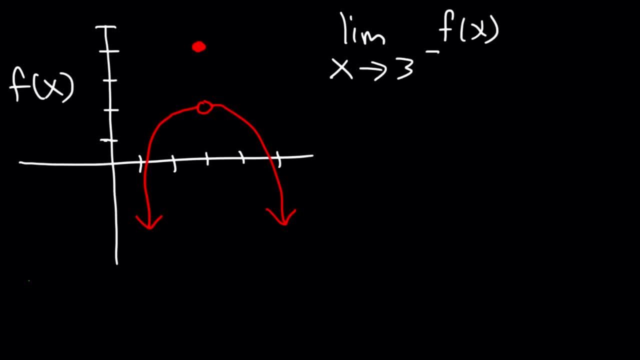 is the graph of f. So here is an x value of 3.. As we approach it from the left side, notice that the y value is 2.. So this is equal to 2.. Now what is the limit as x approaches 3 from the right side. 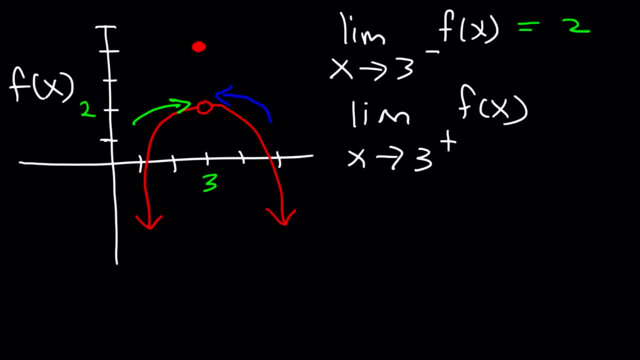 So as we approach an x value of 3 from the right side, the y value is still 2.. Now what is the limit? as x approaches 3 from either side, Because these two values are the same, the limit exists. It's equal to 2.. 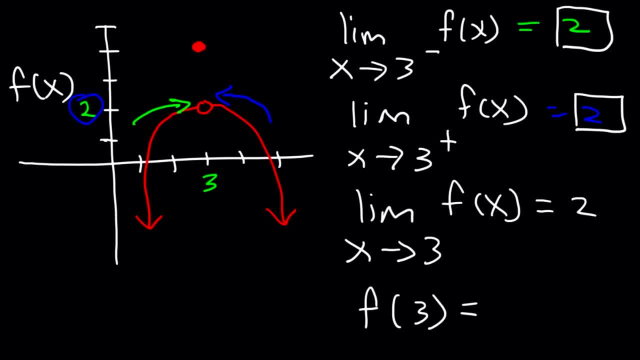 Finally, what is the value of f of 3? When x is exactly 3,, what is the value of y? So whenever you get a question like that, look for the closed circle. The closed circle has a y value of 4.. So f of 3 is equal to 4.. 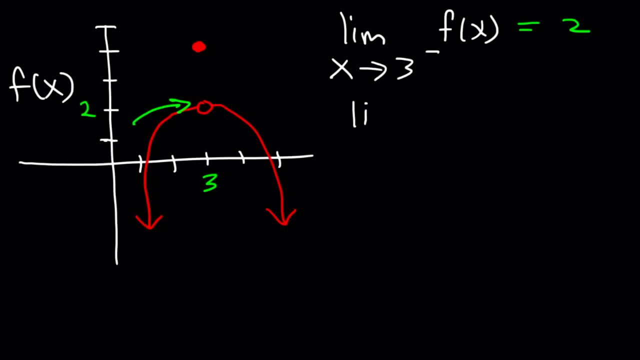 So this is equal to 2.. Now what is the limit as x approaches 3 from the right side? So as we approach an x-value of 3 from the right side, the y-value is still 2.. Now what is the limit as x approaches 3?? 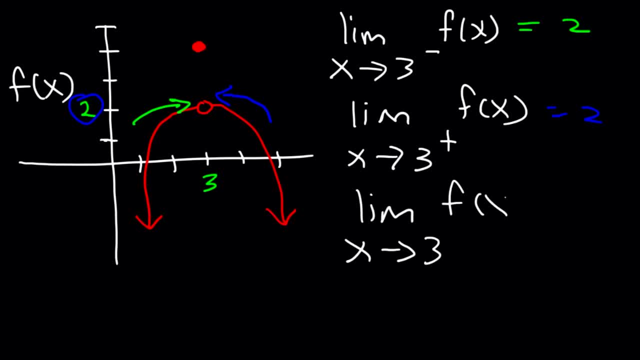 So this is the graph of f. The y-value is 3 from either side. Because these two values are the same, the limit exists. It's equal to 2.. Finally, what is the value of f When x is exactly 3,? what is the value of y? 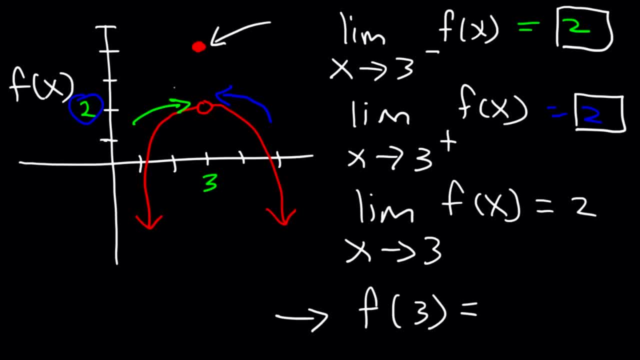 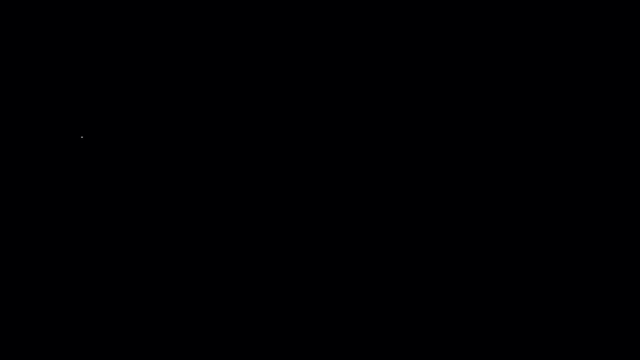 So whenever you get a question like that, look for the closed circle. The closed circle has a y-value of 4.. So f is equal to 4. And it's less than 2. And the positive is opposite 1.. And therefore, what is the它的 limit in terms on its x angle? 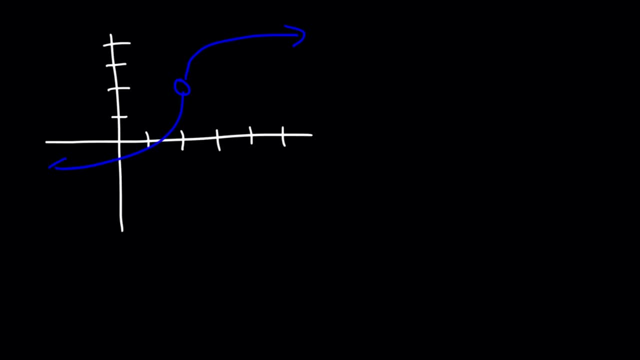 So now it's a big problem. I don't know if you can imagine it. It's a massive calculation of what is its time. Okay, Let's go ahead and plot this. Consider this one. So what is the limit as x approaches 2 from the left side. And what is the limit as x approaches 2 from the right side? Again, I want to go through it. The x is proportional to the indirection to the ones that are correct. So let's subtract x from the value of a And let's subtract 1 as x approaches 1 from the left side. 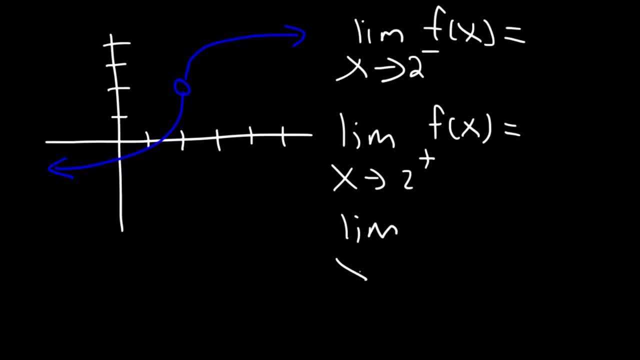 Next we need to write that26 in order to figure out what is the limit. How does thisけど create Salino? We will tell you what that is And then find the limit as x approaches 2 from either side, And, in addition to that, find the value of f of 2.. 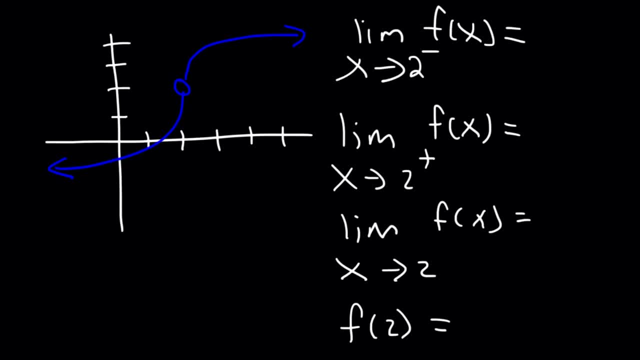 So go ahead and pause the video. Go ahead and find the answers to these problems. So let's start with the first one. So here's an x value of 2.. As we approach that point from the left side, notice that the y value is also 2.. 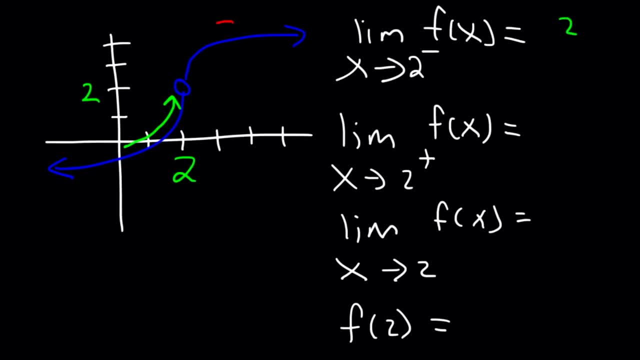 Now, as we approach, x equals 2 from the right side, the y value is still 2.. So therefore, the limit as x approaches 2 from either side must be 2 as well, because the left side and the right side have the same y value. 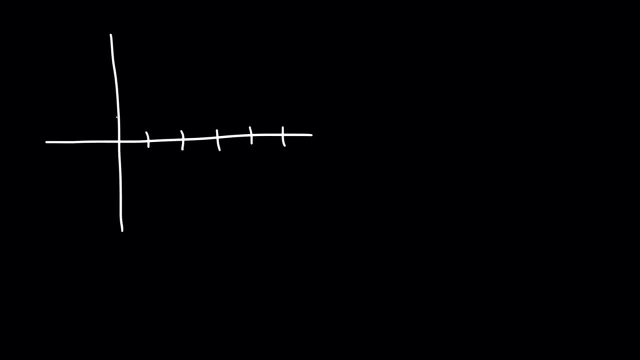 Consider this one. So what is the limit as x approaches 2 from the left side And what is the limit as x approaches 2 from the right side, And then find the limit as x approaches 2 from the left side And then find the limit as x approaches 2 from either side? 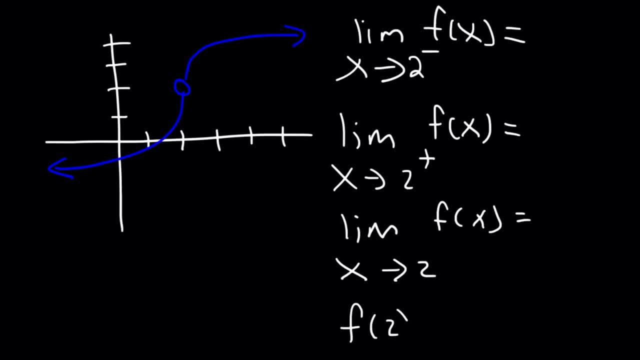 And, in addition to that, find the value of f of 2.. So go ahead and pause the video. Go ahead and find the answers to these problems. So let's start with the first one. So here's an x value of 2.. 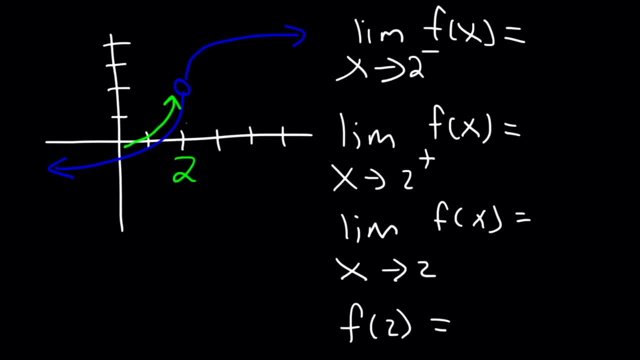 As we approach that point from the left side, notice that the y value is also 2.. Now, as we approach, x equals 2 from the right side, the y value is still 2.. So therefore, the limit as x approaches 2 from either side must be 2 as well, because the left side and the right side have the same y value. 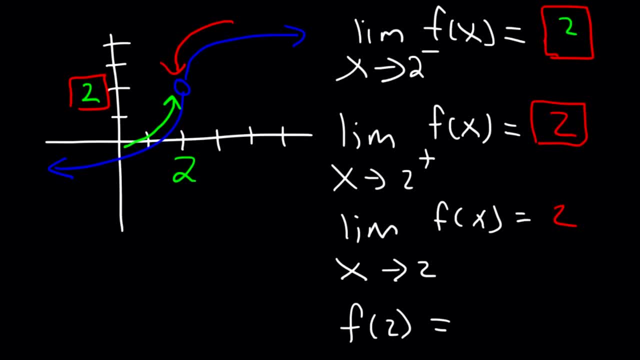 Now, what is the value of f of 2?? So when x is exactly 2, what is the y value? Notice that there's no closed circle in this particular example. So therefore it does not exist. If you don't see a closed circle at x equals 2, f of 2 is not defined. 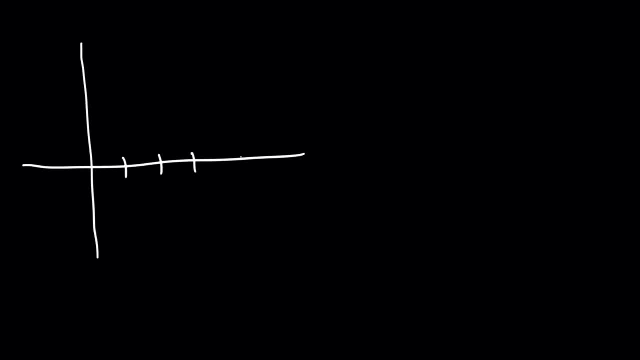 Now let's look at a fourth example. What is the limit as x approaches 4 from the left side, And also find the limit as x approaches 4.. So what is the limit as x approaches 4 from the right side And as x approaches for from either side? 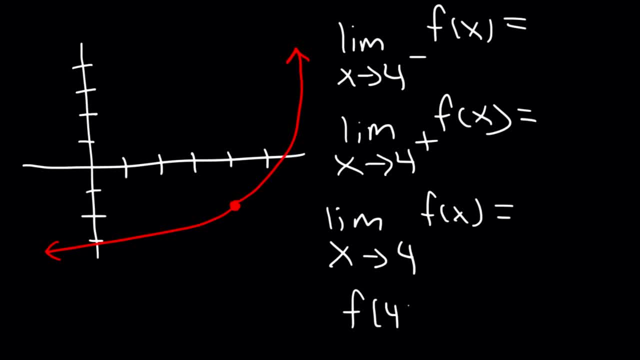 And also find the value of f. So what is the limit as x approaches for from the left? Looking at the graph, here's an x value of 4.. So as we approach from the left side, notice that the y value is approximately negative 2.. 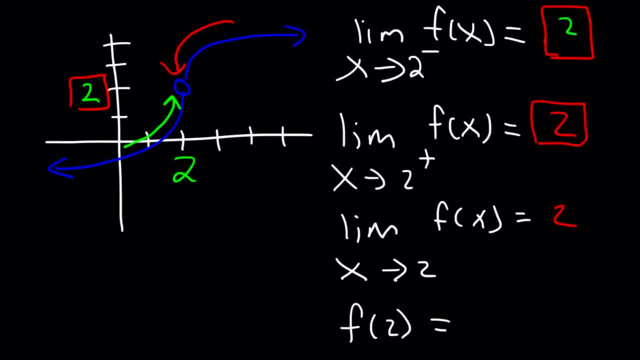 Now, what is the value of f of 2?? So when x is exactly 2, what is the y value? Notice that there's no closed circle in this particular example. So therefore it does not exist. If you don't see a closed circle at x equals 2, f of 2 is not defined. 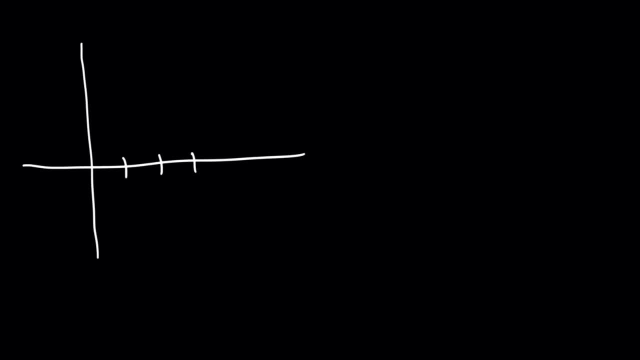 Now let's look at a fourth example. Let's look at a fourth example. What is the limit as x approaches 4 from the left side? And also find the limit as x approaches 4 from the right side And as x approaches 4 from either side. 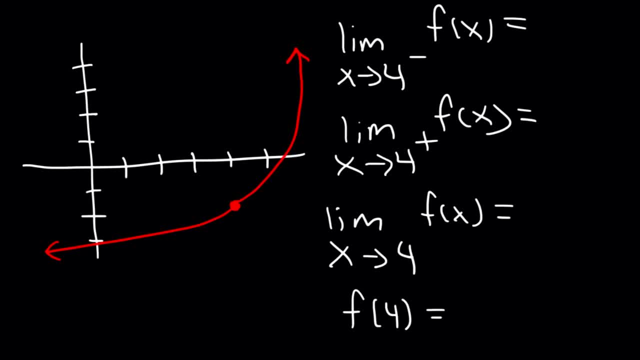 And also find the value of f of 4.. So what is the limit as x approaches 4 from the left? Looking at the graph, here's an x value of 4.. So as we approach it from the left side, notice that the y value is. 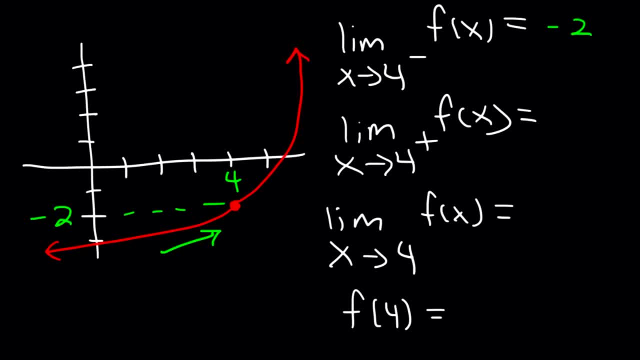 approximately negative 2.. Now, as we approach positive 4 from the right side, the y value is still negative 2. So the limit exists, Since the left side is the same as the right side. the limit as x approaches 4. 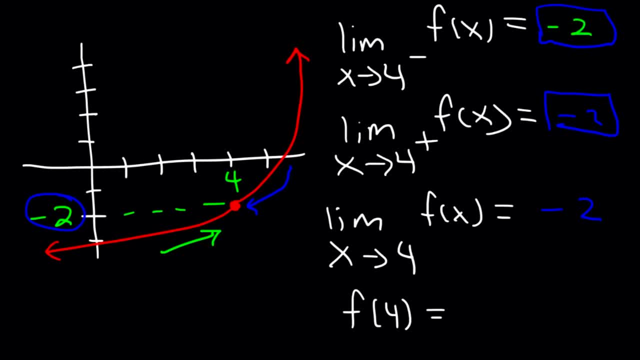 from either side is also negative 2.. Now what about f of 4?? Notice that we do have a closed circle at x equals 4.. So it's also equal to negative 2.. So therefore, everything is the same. The function is continuous at an x value of 4.. 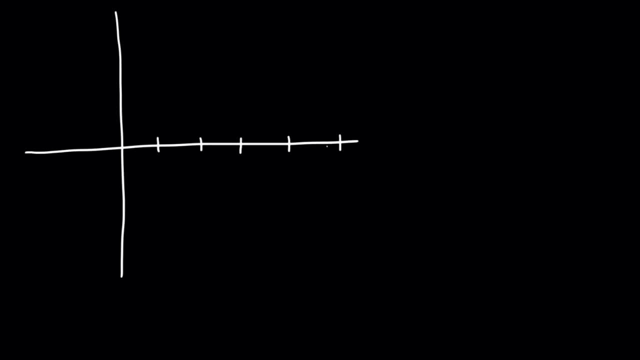 Here's another problem that you can try. Here's another problem that you can try. So what is the limit? as x approaches 4 from the left side, X is negative 4.. Then you have x over 3 from the left side. 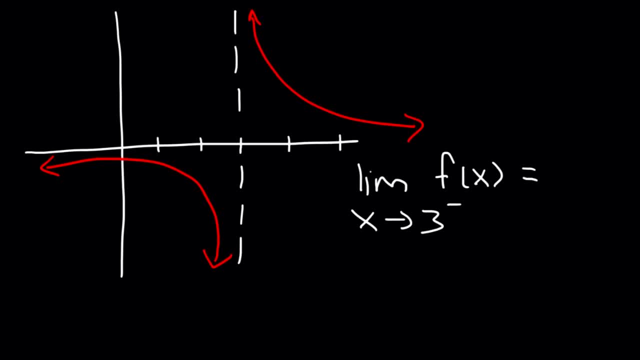 Let's start with that. So what do you think it is equal to Here's 3.. It's the vertical asymptote. As we follow the curve, as we approach 3 from the left side, notice that it does not converge to a specific value. 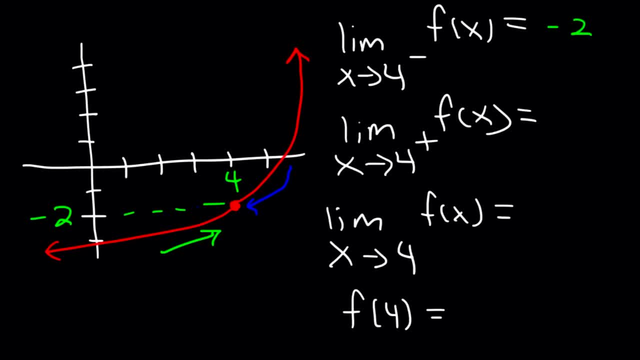 1. Now, as we approach positive 4 from the right side, it does also designate us toología 1. the y-value is still negative 2. So the limit exists, Since the left side is the same as the right side. the limit as x approaches 4 from either side is also. 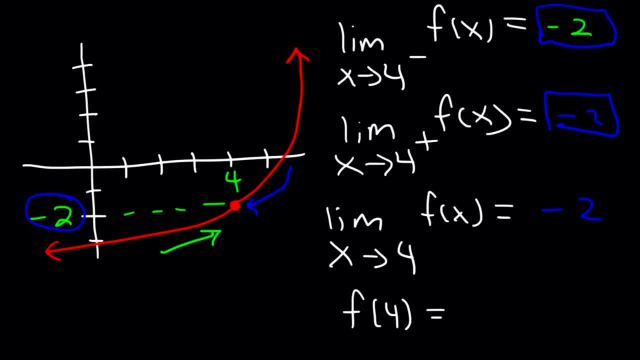 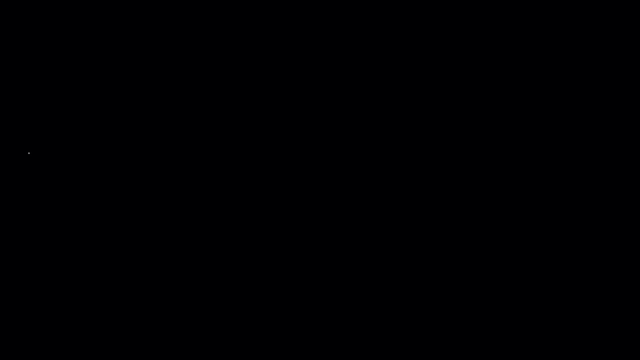 negative 2.. Now what about f of 4?? Notice that we do have a closed circle at x equals 4, so it's also equal to negative 2.. So therefore, everything is the same. The function is continuous at an x value of 4.. 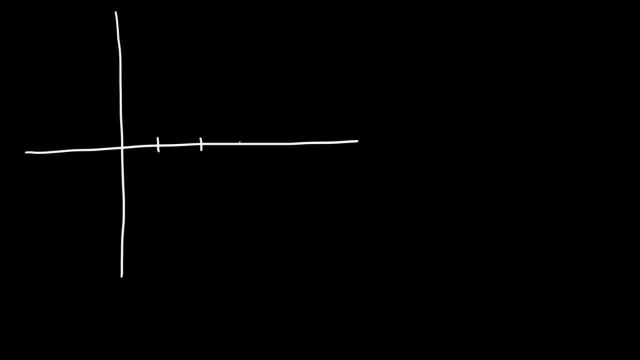 Here's another problem that you can try. So what is the limit as x approaches 3 from the left side? Let's start with that. So what do you think it's equal to? So what is the limit as x approaches 3 from the left side? Let's start with that. 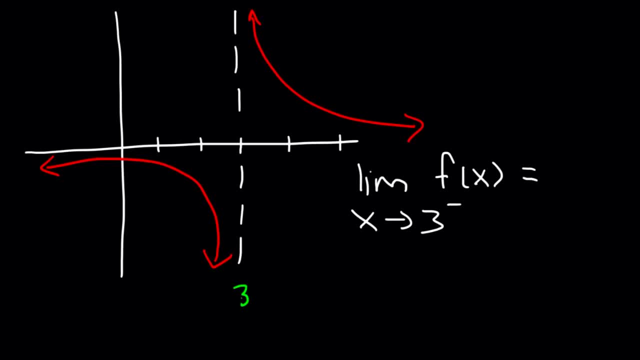 So here's 3.. It's the vertical asymptote And as we follow the curve, as we approach 3 from the left side, notice that it doesn't converge to a specific y-value. It keeps getting lower and lower and lower. So therefore it goes to. 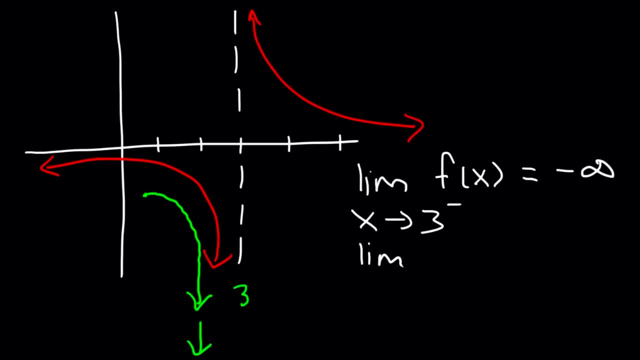 negative infinity. Now what about the limit as x approaches 3 from the right side? If we follow the curve towards the vertical asymptote with an x value of 3,. if we follow the curve towards the vertical asymptote with an x value of 3,. 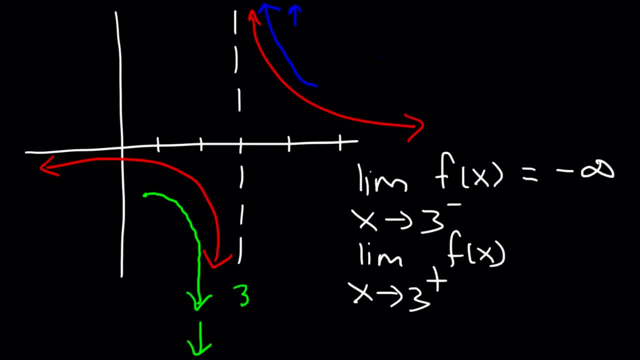 notice that keeps going higher and higher and higher. So therefore it approaches positive infinity. Now, what is the limit? as x approaches 3 from either side, Because these two do not match, the limit does not exist. Now what about f of 3?? 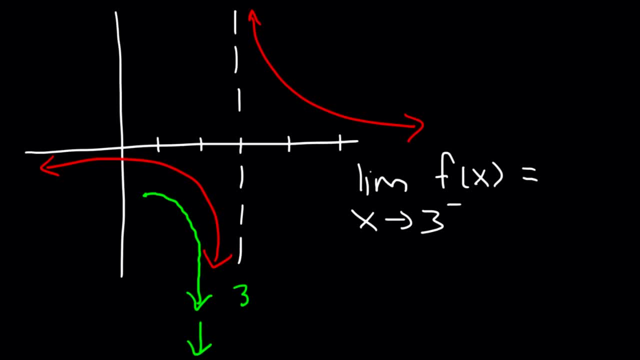 It keeps getting lower and lower and lower. Therefore it goes to negative infinity. Now, if we take a look at the limit, as x approaches 4 from the right side, there will be no y. Then it noticed it was going to be 3, itslış, it didn't have to clean up. 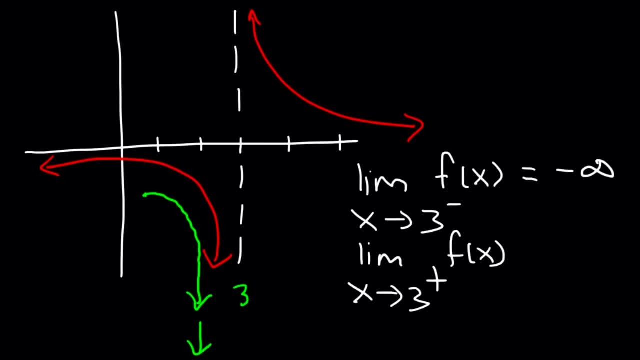 So instead we'll put 3 in side. If we follow the curve towards the vertical asymptote with an x value of 3, notice that it keeps going higher and higher and higher. So therefore it approaches positive infinity. Now what is the limit? as x approaches 3, from either 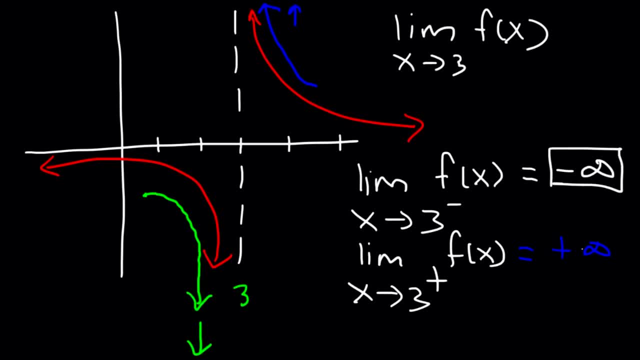 side, Because these two do not match, the limit does not exist. Now what about f of 3?? We don't have any closed circle at x equals 3, so therefore, f of 3 is not defined, It doesn't exist. 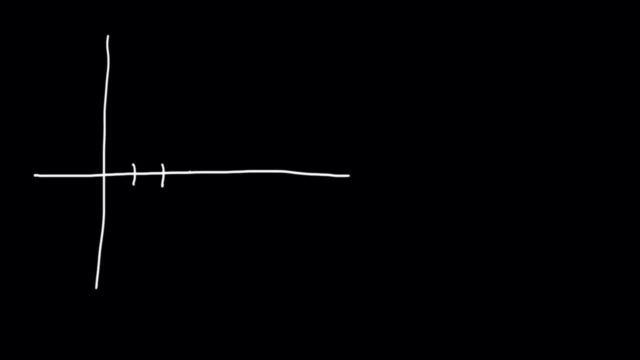 Let's try another similar example. What is the limit as x approaches? positive 4 from the left side, given the graph of f of x. So here is the x value of 4, and as we approach it, notice that the curve increases. It keeps getting higher and higher, So the y value. 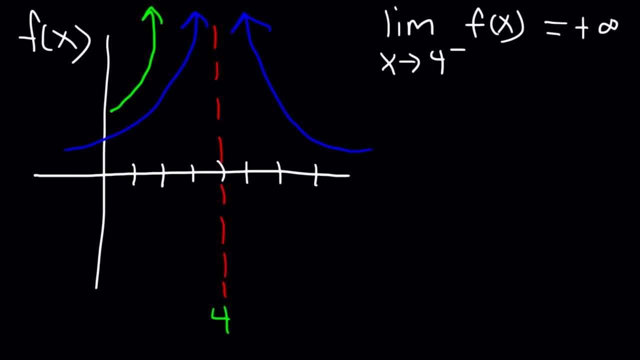 approaches infinity, That is, positive infinity. Now, as we analyze the limit as x approaches 4 from the right side, as we follow the curve towards positive 4 from the right, it also keeps going higher and higher. It goes towards positive infinity. So, therefore, what is the limit as x? 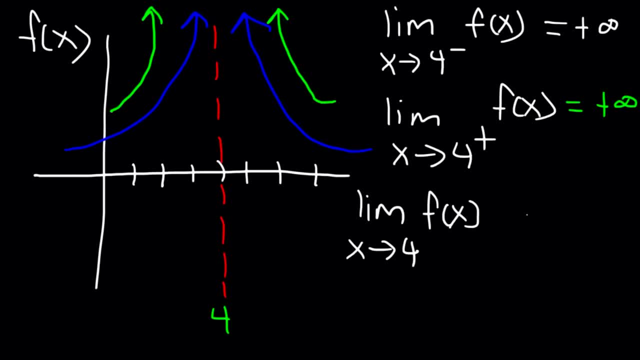 approaches 4 from either side. Since these two are the same, you can see that it approaches positive infinity. Now, granted, infinity is not really a number. I mean you can. infinity could be a million, a billion, a trillion, or just. 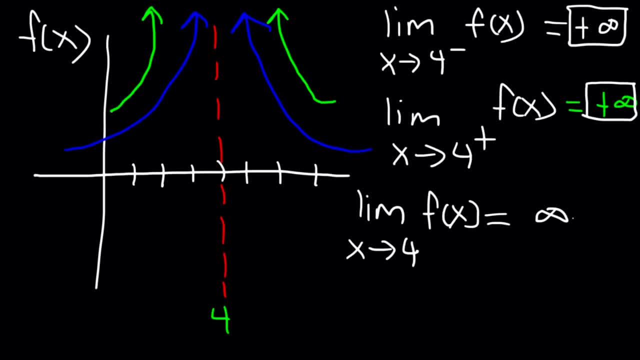 something that's just it's and never ending. it's just keep increasing. So, because it has a conversion of specific value, you could also say that this limit does not exist. Some textbooks will have this answer. some will have infinity. so infinity really doesn't exist. It's just a way of describing what happens. as x. 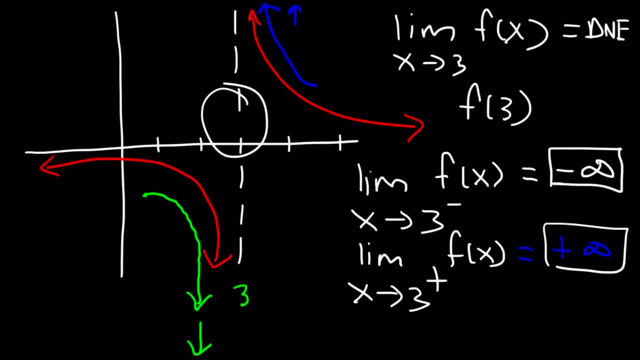 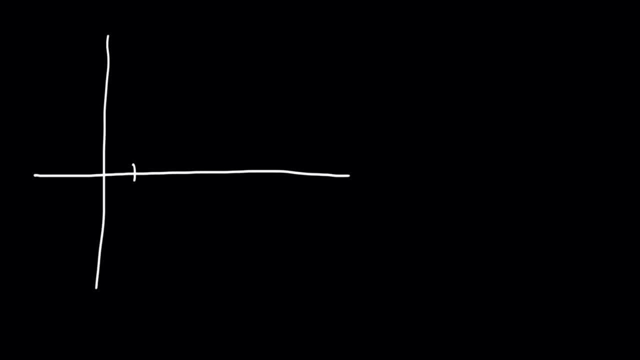 We don't have any closed circle at x equals 3, so therefore f of 3 is not defined, it doesn't exist. Let's try another similar example. What is the limit as X approaches positive 4 from the left side, given the graph of f of X? 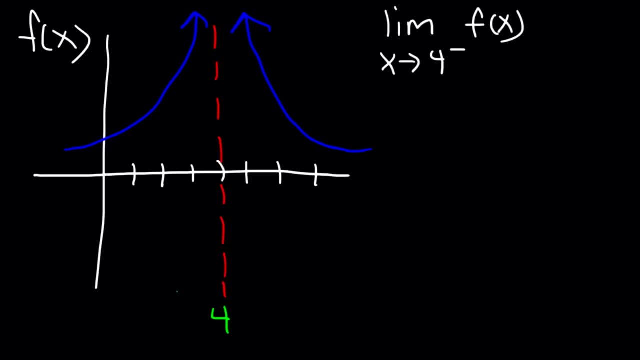 So here's the X value of 4.. And as we approach it, notice that the curve increases. It keeps getting higher and higher. So the Y value approaches infinity, That is positive infinity. Now, as we analyze the limit, as X approaches 4 from the right side, 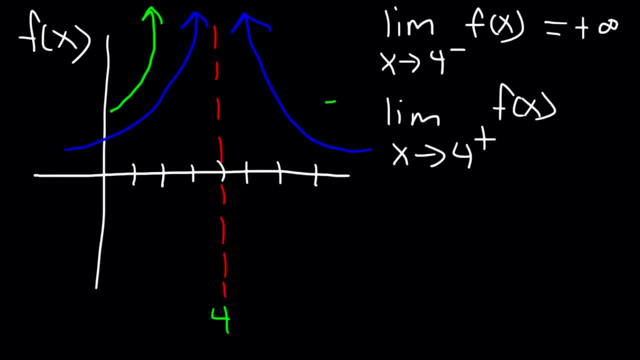 as we follow that, we follow the curve towards positive 4 from the right. it also keeps going higher and higher. It goes towards positive infinity. So therefore, what is the limit as X approaches 4 from either side, Since these two are the same? 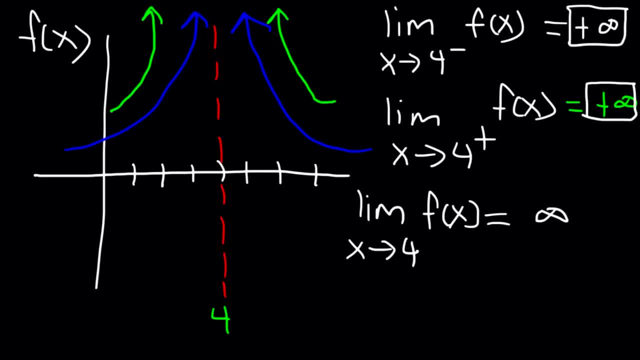 you can see that it approaches positive infinity. Now, granted, infinity is not really a number. Infinity could be a million, a billion, a trillion or just something. that's just, it's a never-ending, it's just keep increasing. So, because it doesn't converge to a specific value, 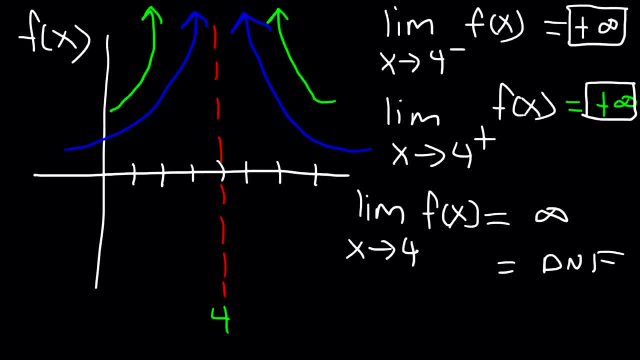 you could also say that this limit does not exist. Some textbooks will have this answer. some will have infinity. So infinity really doesn't exist. It's just a way of describing what happens as X approaches 4.. That is, the curve gets bigger and bigger and bigger. 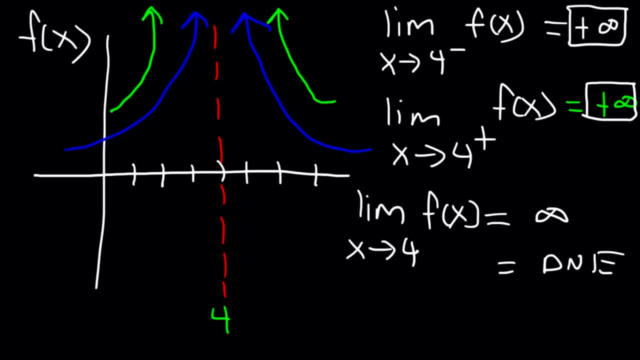 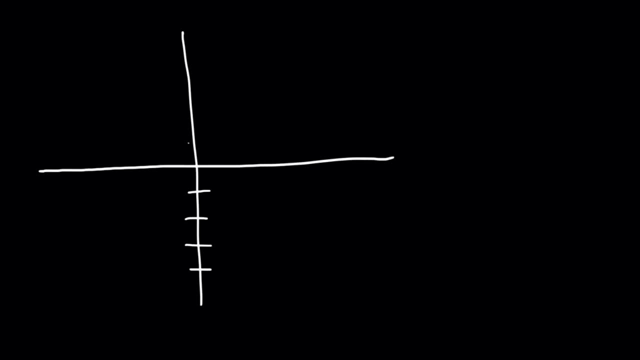 The Y value, that is, It gets higher and higher and higher. And we know that F is undefined, It doesn't exist. We don't have a closed circle at X equals 4.. Now let's work on some examples with horizontal asymptotes.